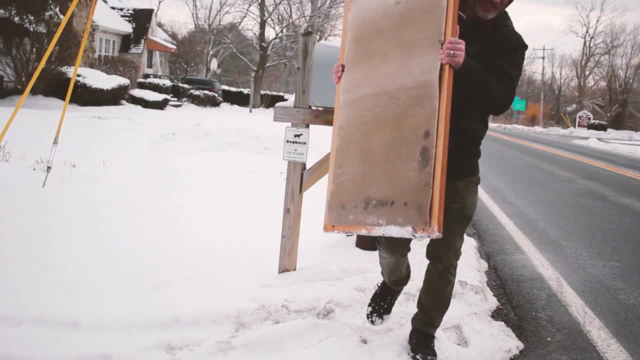 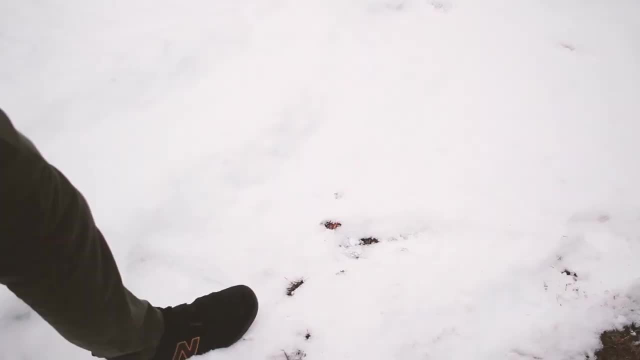 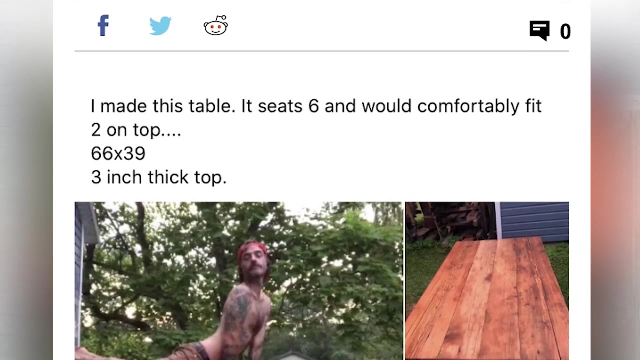 Here's my favorite woodworking project to make and sell on Facebook Marketplace for a quick buck. I've been selling woodworking projects on Facebook Marketplace for years. I even ended up in the newspaper and on the news for my strange selling techniques. Anyway, I found that the one thing that always seems to sell on Facebook Marketplace is mirrors. 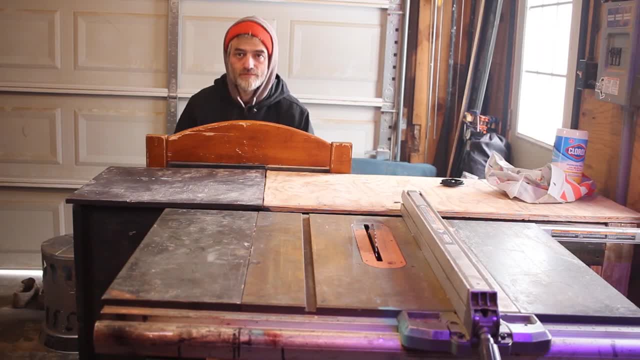 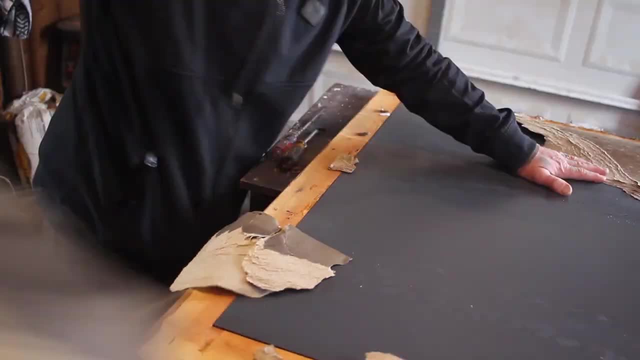 And you can find a mirror on the side of the road pretty much anywhere. Just keep your eye out and you'll find one. I brought this mirror into my workshop and tore the back off of it And removed the mirror from this frame. I'll be saving the wood from this frame for another project down the road. 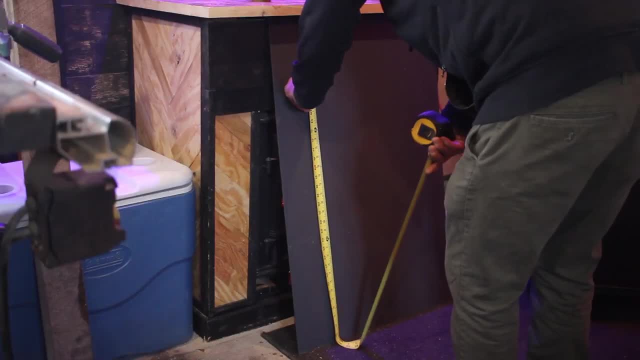 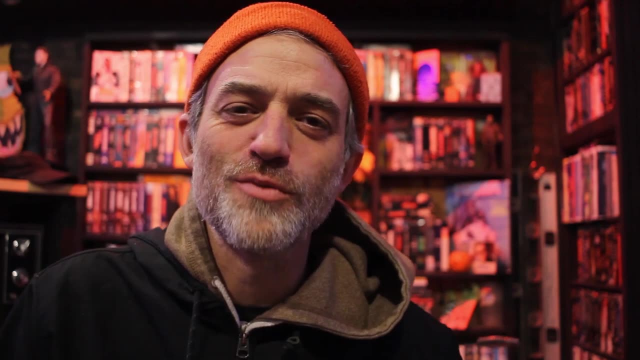 I couldn't find my safety glasses anywhere, So I decided I'd just cut these pieces of wood with my eyes closed to make sure my eyes were safe. I'm kidding, I definitely didn't do that. Don't cut things with your eyes closed. 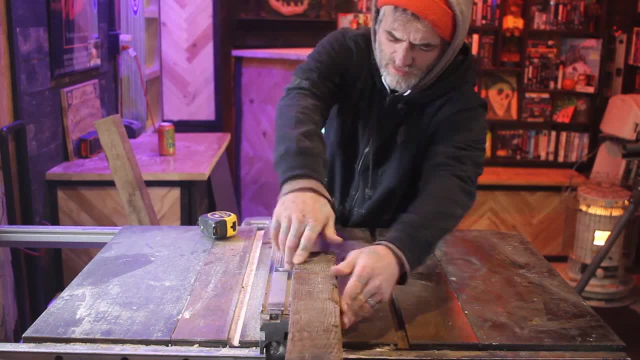 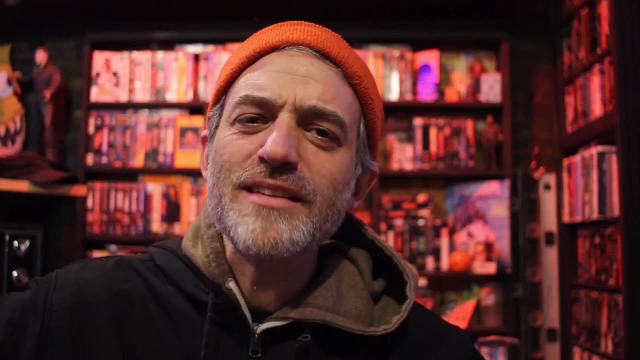 But I actually couldn't find my safety glasses, So I had to build this whole project without them. I know not my smartest decision, But you know these things happen. Leave a comment. Do you guys always wear your safety glasses if you can't find them? 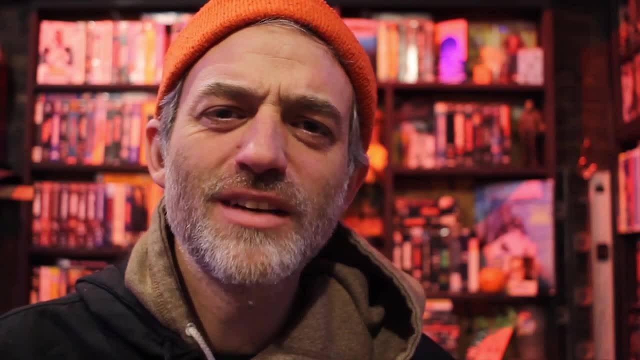 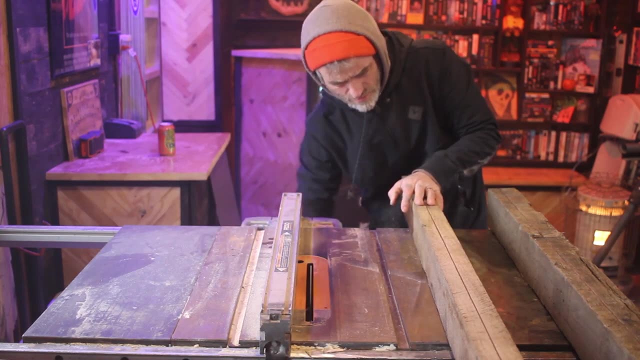 Be honest, I know this is how accidents happen. Rushing, Stuck my finger right into the table. saw one day. Okay, back to the project. So far, all I've done is measure my mirror and start breaking down this wood to build the frame. 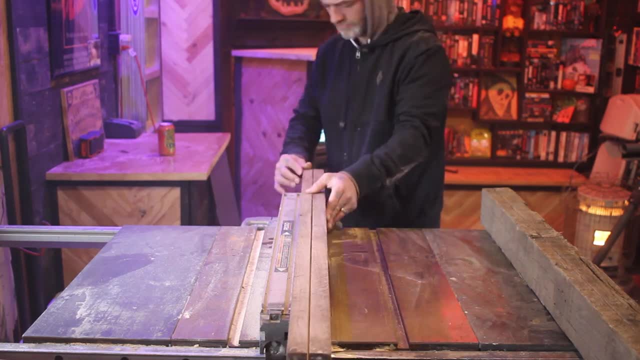 These boards I was using were 4x4's, so I had to rip them on the table saw And to do this I raised the blade a little bit at a time, Passing it through the table saw and flipping the board end to end. 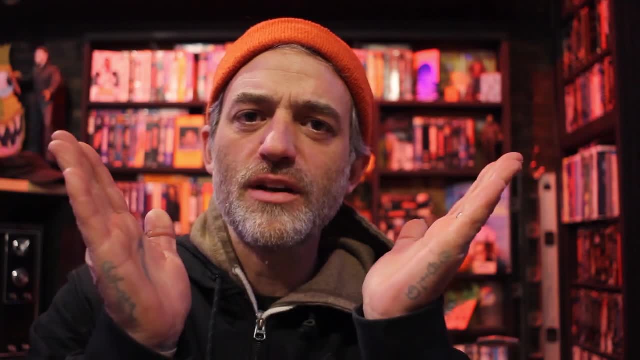 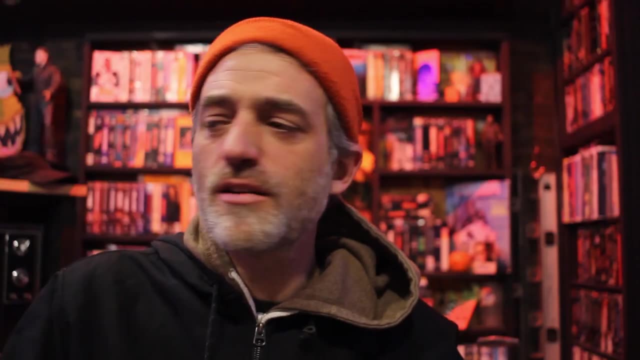 And passing it through again so that I could split the board right down the middle. I would not be able to cut All the way through these boards with one pass, First of all because my blade doesn't go that high And second of all because the saw is not strong enough to cut through that much wood all at once. 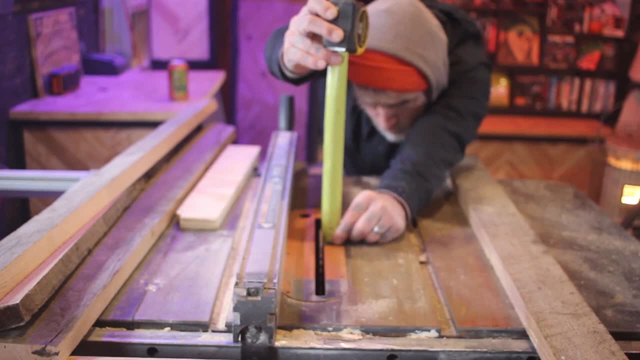 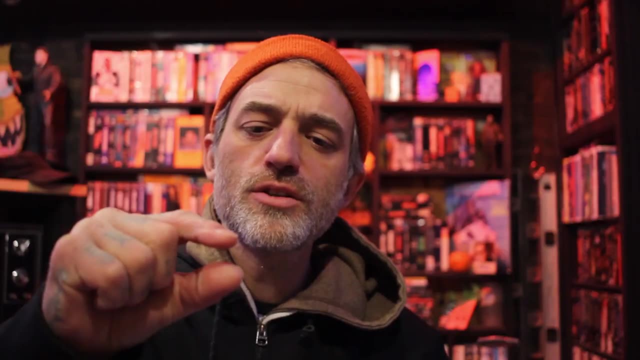 After I had my boards ready to go for the frame, I cut a channel where my mirror itself will be sitting inside the frame. To do this, I raised my blade to a quarter inch- Quarter inch, Yeah- And moved my fence on my table, saw over to a quarter inch as well. 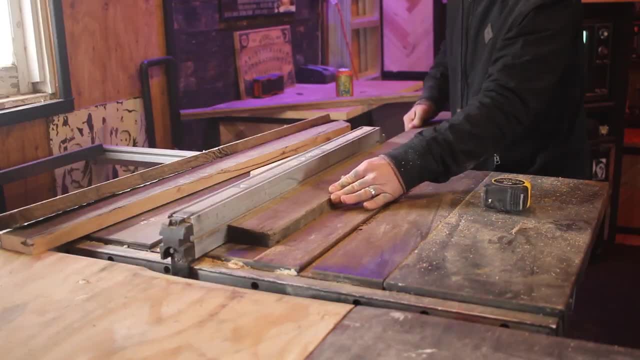 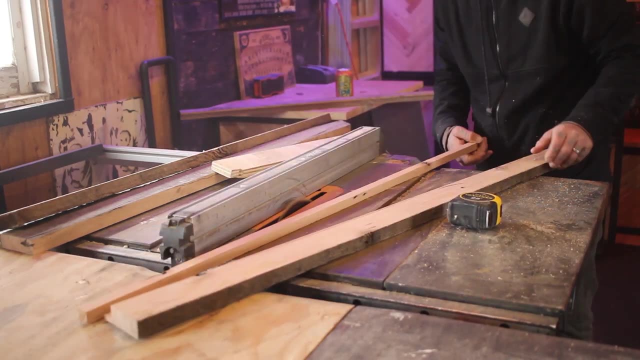 I ran my boards through the blade Laying down. Then I can turn the board up on it's side and run it through, standing up on it's side against the fence, And by making these two cuts you'll remove a quarter inch square along the whole length of your piece of wood.